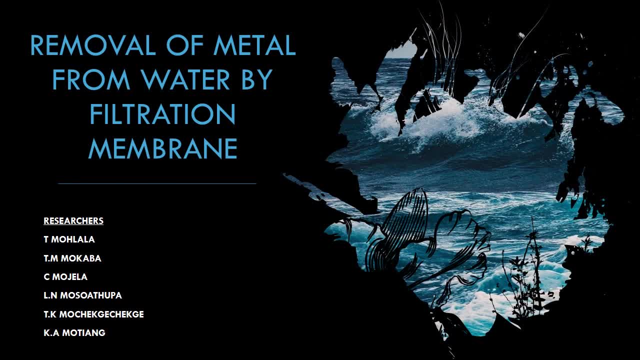 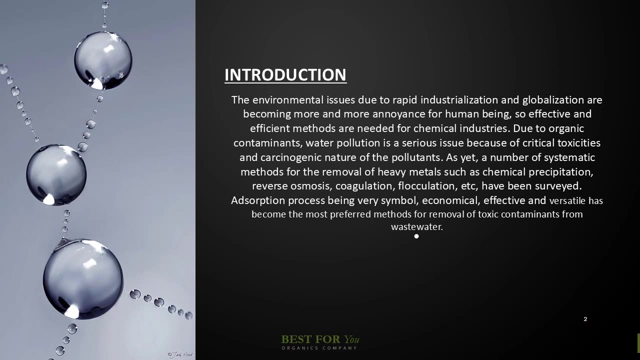 Hello, good people, thank you for joining us on this YouTube channel. Today we'll be talking about the removal of metal from water by filtration membrane. The introduction. The environmental issues due to rapid industrialization and globalization are becoming more and more annoying for human beings. 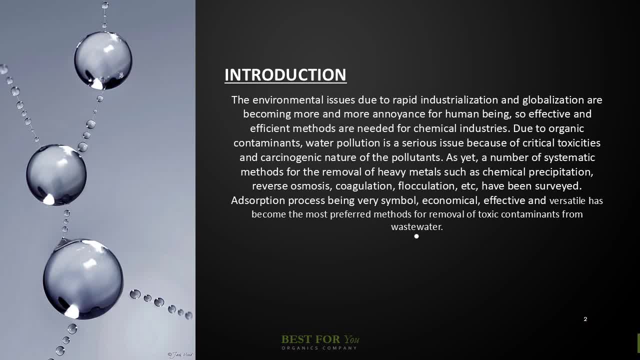 So effective and efficient methods are needed for chemical industries. Due to organic contaminants, water pollution is a serious issue because of critical toxicities and carcinogenic nature of the pollutants. As yet, a number of systematic methods for the removal of heavy metals, such as chemical precipitation, reverse osmosis, coagulation, flocculation, etc. have been surveyed. 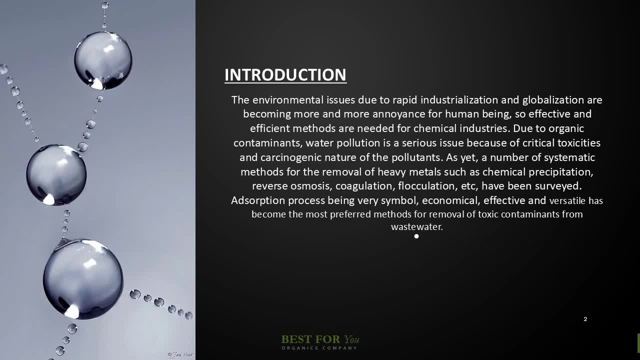 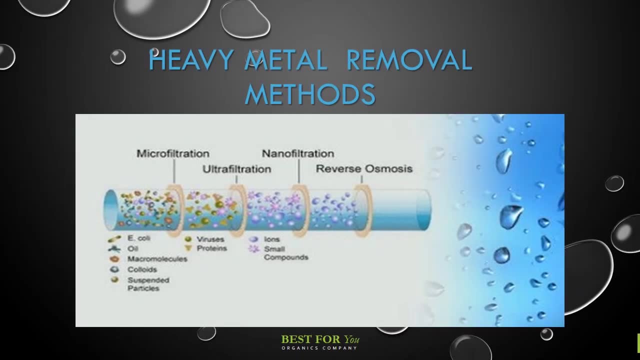 Absorption process, being very simple, Therefore economical, effective and versatile, has become the most preferred method for removal of toxic contaminants for waste water: Heavy metal removal methods. Right here we see a series of steps where water has to go through in order to be clean. 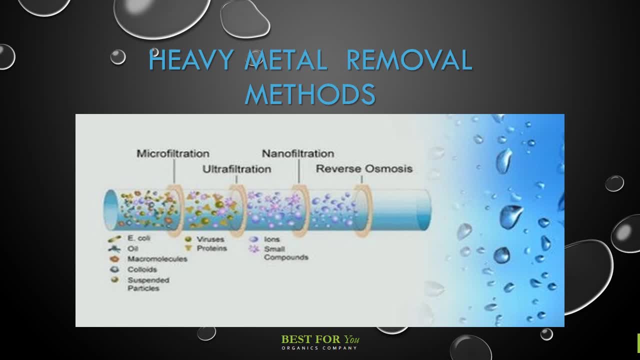 Starting from microfiltration, going down to ultrafiltration, nanofiltration and then we have reverse osmosis In microfiltration. this is where macromolecules are being removed. In ultrafiltration, micro molecules are being removed like viruses and bacteria. 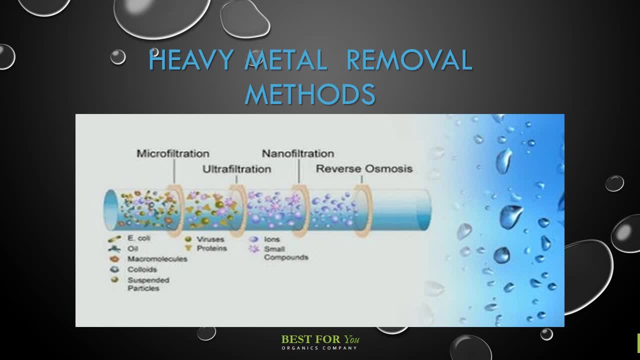 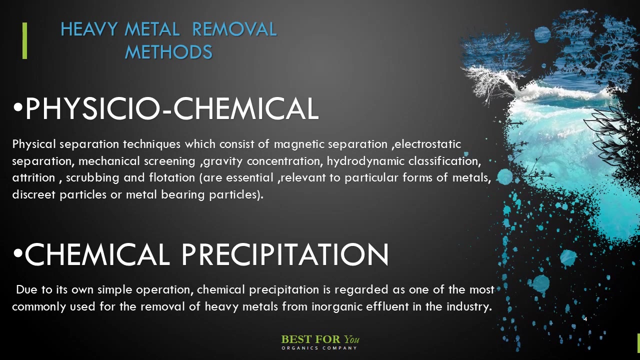 Going to nanofiltration: ions and small compounds are being removed, and then reverse osmosis is where salts and color are being removed. There are four heavy metal removal methods, namely physical-chemical. In physical-chemical physical separation techniques, which consist of magnetic separation, electrostatic separation, mechanical screening, gravity concentration, hydrodynamic classification, attrition, scrubbing and flotation are essential relevant to particular forms of metals, discrete particles or metal-bearing particles. 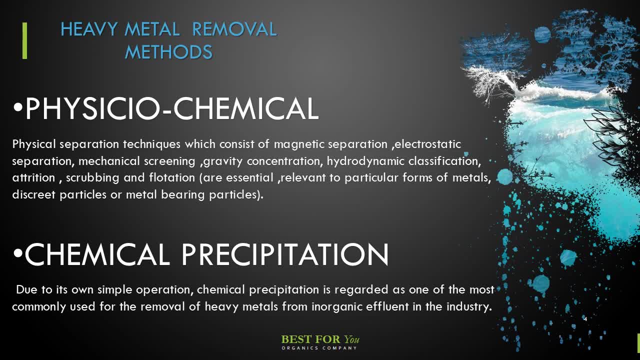 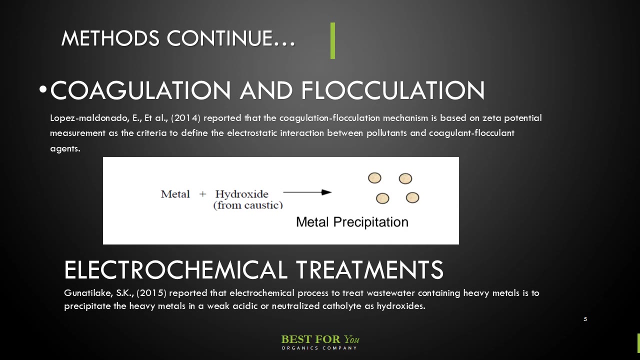 We then have chemical precipitation in which, due to its own simple operation, chemical precipitation is one of the most commonly used of all the heavy metals and minerals in the industry. The third method would be coagulation and flocculation, which was reported that coagulation and flocculation might are matched with milonder. 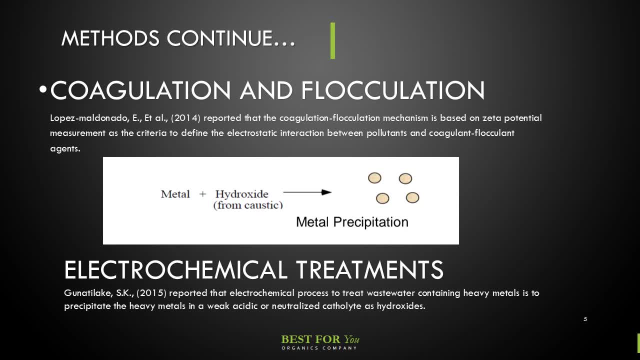 In other words, the last loading ofCHRs is based on zeta potential measurements as the criteria to define the electrostatic interactions between pollutants and coagulant flocculant agents. right here we will see the mechanism. fourth method is electrochemical treatment, which was reported that electrochemical process to treat 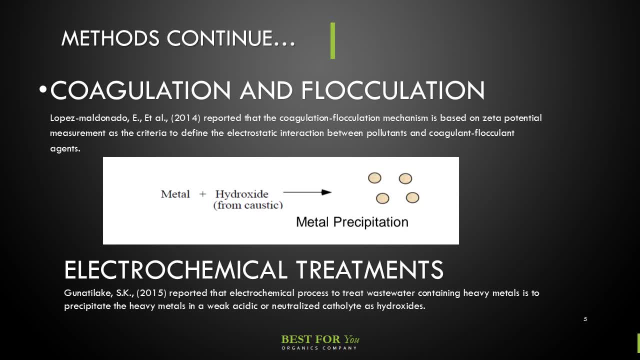 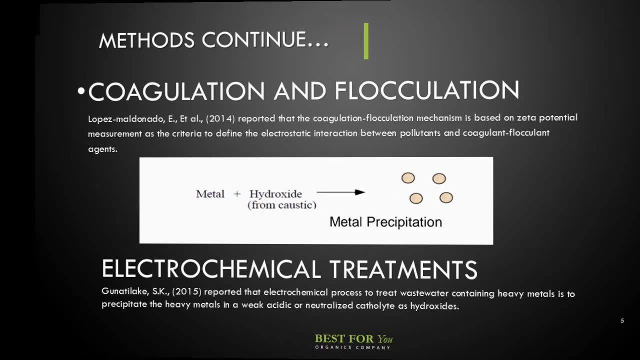 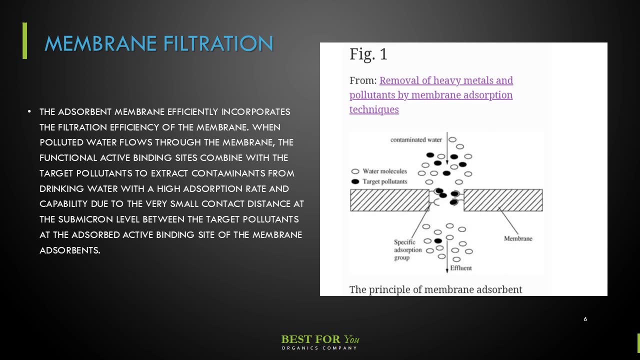 wastewater containing heavy metals is to precipitate the heavy metals in a weak acidic or neutralized catecholitis or hydroxide. the membrane filtration- the absorbent membrane- efficiently incorporates the filtration efficiency of the membrane. when the polluted water flows through the membrane, the functional active binding sites combine with the target pollutants to 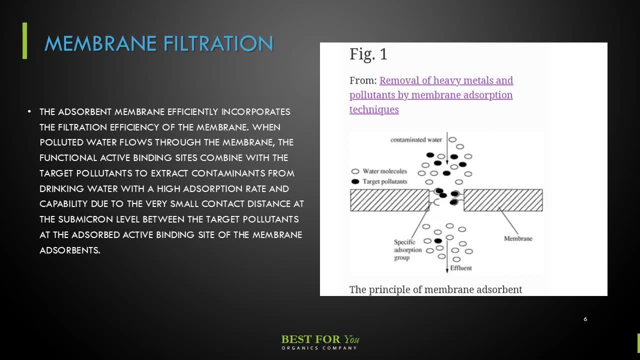 extract contaminants from the drinking water with a high absorption rate and capability of the water to absorb the pollutants. and the ability of the water to absorb the pollutants due to the very small contact distance at the submicron level between the target pollutants at the adsorbed active binding sites of the membrane adsorbent. 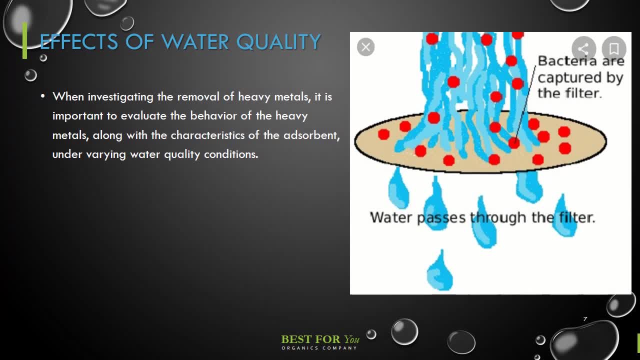 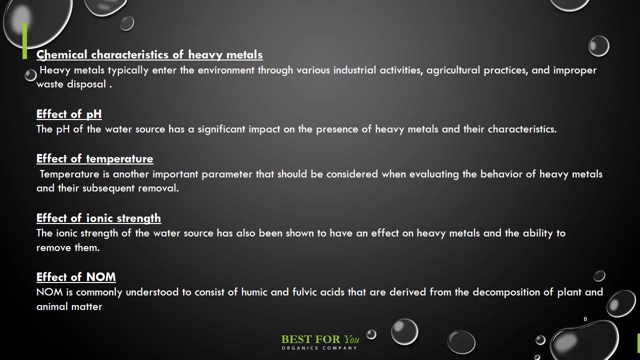 effects of water quality. when investigating the removal of heavy metals, it is important to evaluate the behavior of the heavy metals, along with the characteristics of the adsorbent and a varying water quality conditions. many effects of water include the chemical characteristics of metals, effects of pH, effects of temperature, effects of ionic strength and effects of norm. 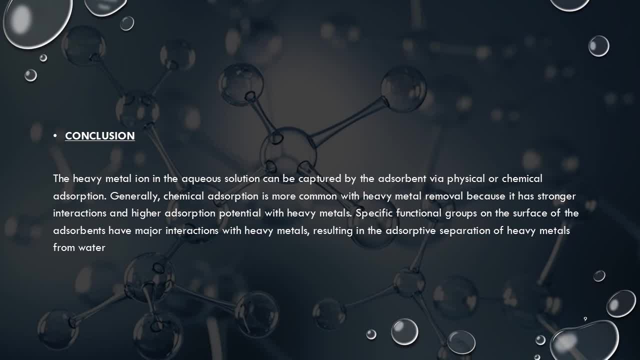 in conclusion, the heavy metal iron in the aqua solution can be captured by the adsorbent via physical or chemical adsorption of the liquid metal and water. it is important to analyze the Generally, chemical adsorption is more common with heavy metal removal because it has stronger